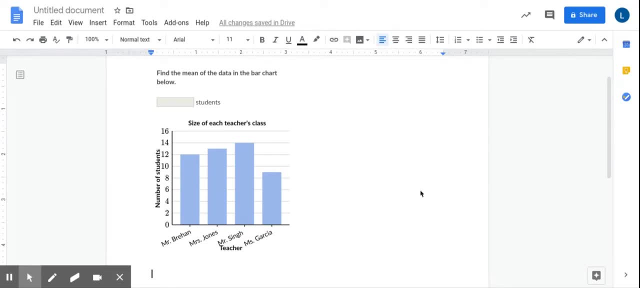 Good morning. this is Miss Moore. I just wanted to work through a couple of problems with you that represent data in different ways. So this is a bar chart and we're gonna find the mean by looking at the bar chart. So right here we have. 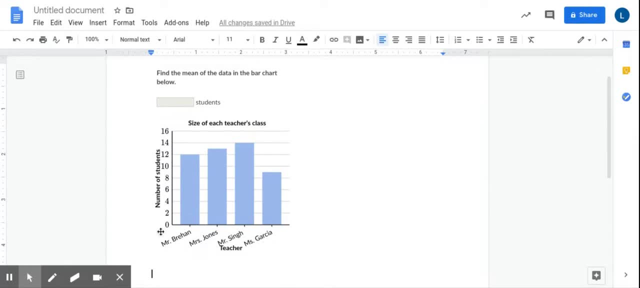 four different classes, four different teachers, and it shows their class size for one of their classes. So to find the mean, we know that we have to add all of the numbers together and then divide it by the number of numbers present. So, for example, Mr Brennan has 12 students in his class. I apologize for. 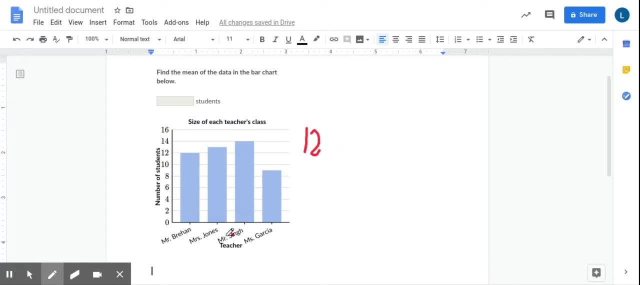 my handwriting. it's really hard to write with a mouse. We're gonna add that to Miss Jones' class of looks like she has 13.. And then Mr Singh has 14 students And we're gonna add Miss Garcia has nine. 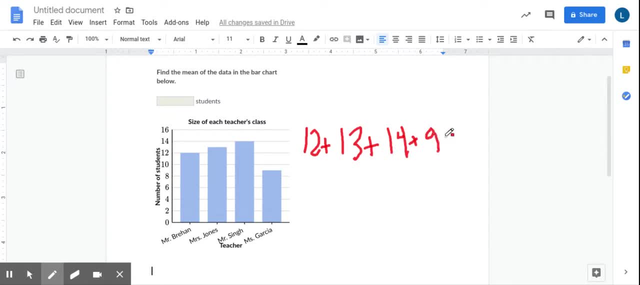 students. So the first step to finding the mean is to add all of those together. When we do that, we get 48 students total, And then if we wanted to find the average class size, we would have to take the total number of students and divide it by how many classes there are. So we're. 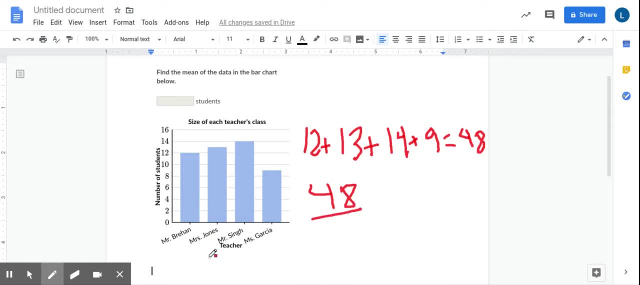 gonna do 48 divided by Mr Brennan, Miss Jones, Mr Singh and Miss Garcia. That's four different teachers representing four different classes. Oops And eraser, Sorry. Okay. so 48 divided by four will give us 12 students per class. So that means if: 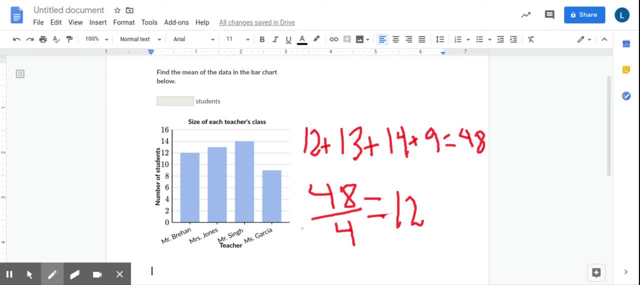 all of the classes were added up all together and then the students were distributed so that each class had the same amount of students. there will be 12 students in each class.